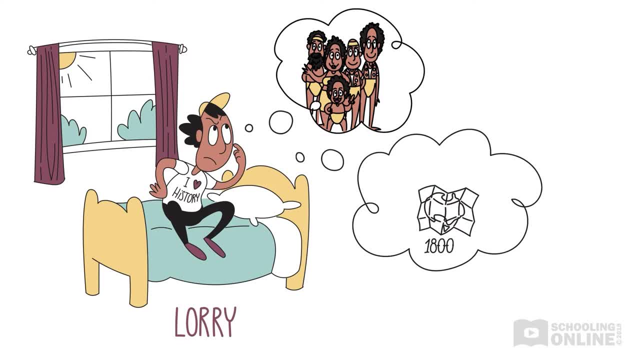 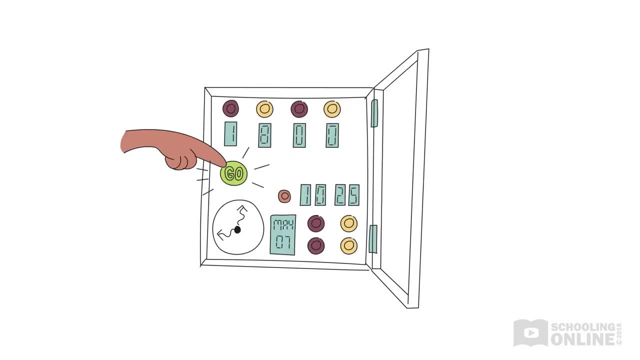 He decides that he wants to learn about what life was like in Australia in the 1800s, 200 years ago. With as much courage as he can muster, he decides to go to Australia In the summer. Laurie presses down on the big green: go button. 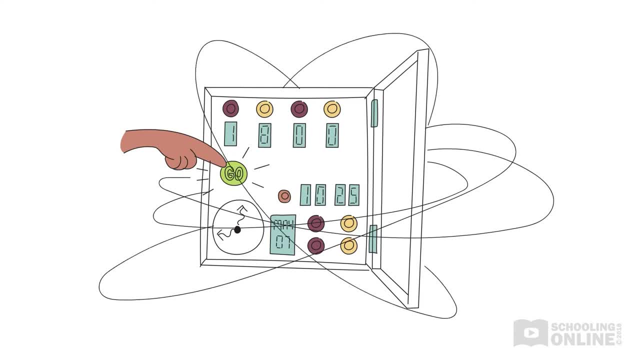 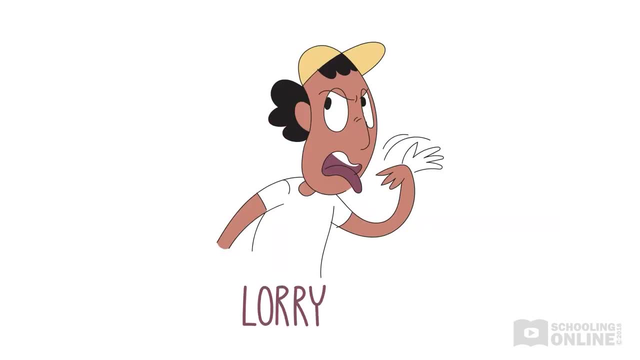 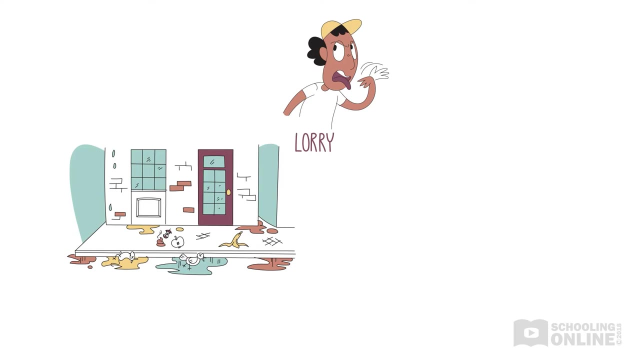 Wind whips through his hair as his room begins to fade and Laurie shuts his eyes in fear. Suddenly, Laurie's nostrils are filled with an overwhelmingly putrid smell. Although he doesn't know it, there were no sewerage systems in the 1800s. 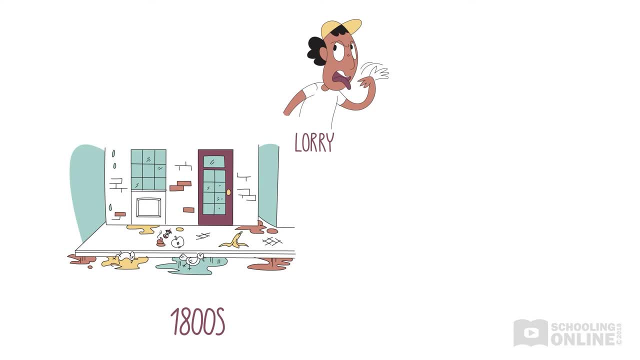 Consequently, animal droppings, old food and dead rats littered the streets, making them smell terrible. Now Laurie can smell these disgusting odours. It is nothing like the crisp clean air back home in the 21st century. Laurie slowly opens his eyes. 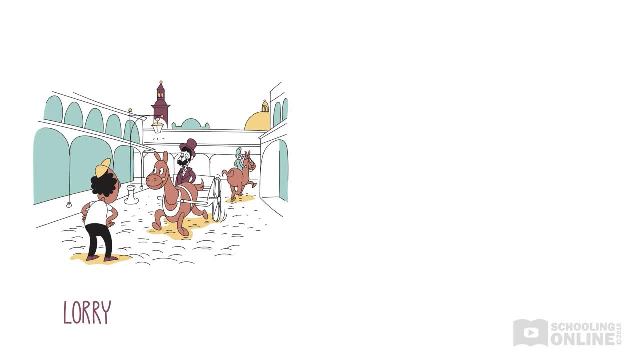 In front of him lies a wide, dusty street. A horse trots towards Laurie, pulling behind it a man in a cart. Cool Laurie, thinks to himself. Cars had not been invented. They weren't invented by the 1800s, nor planes. 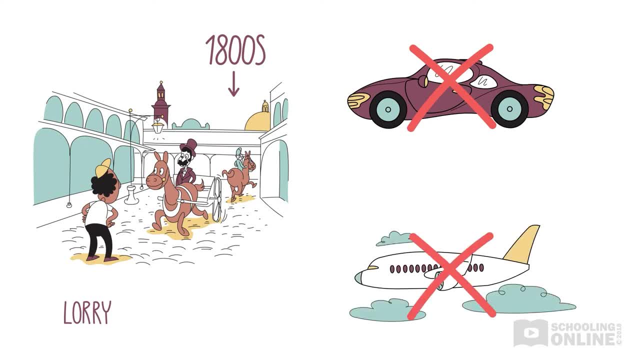 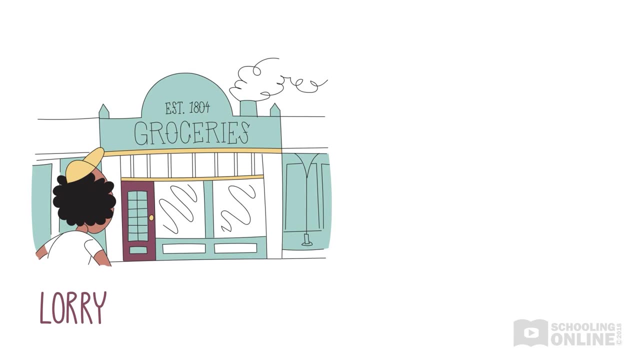 To travel to different places. men and women rode horses and took trains. I guess you couldn't travel very far if you lived in the 1800s, Laurie deduces. Laurie is feeling a little bit sick now from the bad smells in the street. 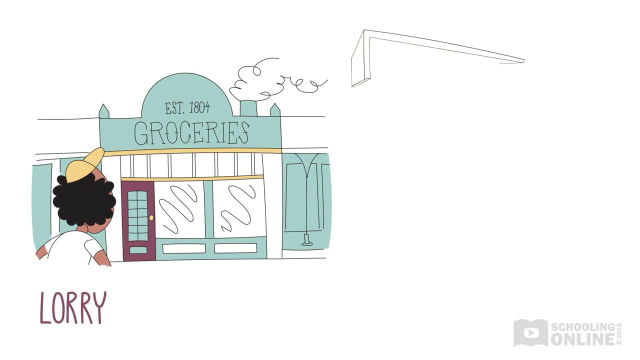 so he decides to explore the shop closest to him- a grocer. We still have grocery shops like Woolies in the 21st century. Laurie exclaims excitedly. But our grocery shops look very different to this one. The shop is painted white and has two big windows at the front. 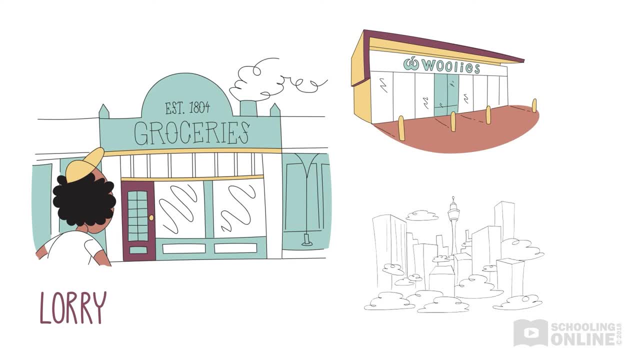 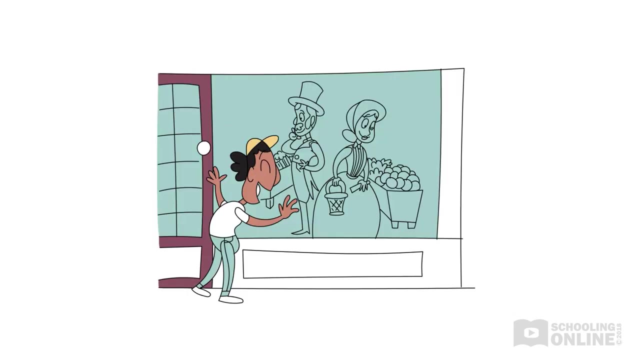 and a chimney on top, puffing smoke from a wood fire, Unlike in the 21st century, where skyscrapers tower overhead. there weren't very many shops in the 1800s and they weren't very big. Peering through the window, Laurie watches a man and woman.